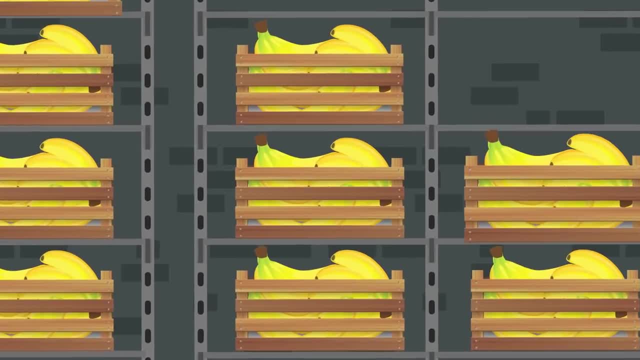 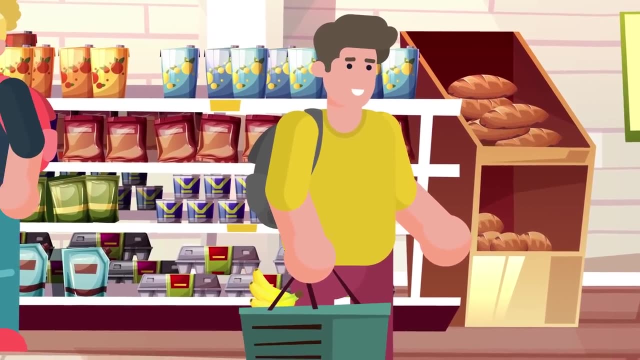 its name because it travels from place to place to find food rather than building a web. It's also known as the Banana Spider because of its propensity for hiding in yellow fruit. It can be found in South and Central American countries. Occasionally, it ends up in England or America. 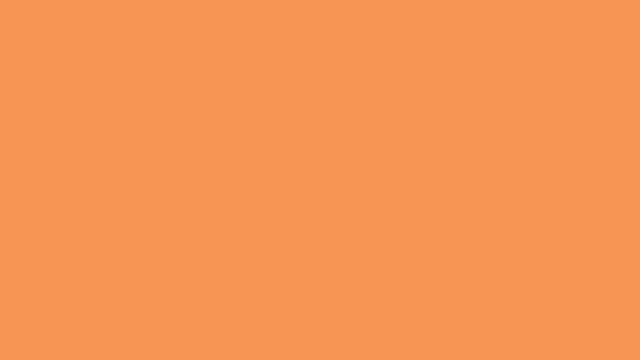 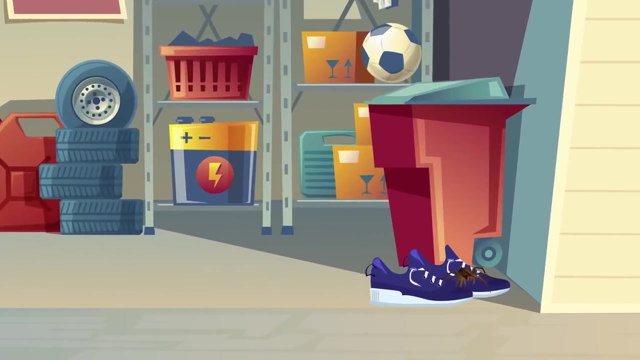 showing up as a horrid surprise for someone purchasing a bunch of bananas, While the Brazilian Wandering Spiders nest on the ground in the forest, they also like hiding in dark, moist places such as piled logs, garages, shoes and closets As a defense mechanism. 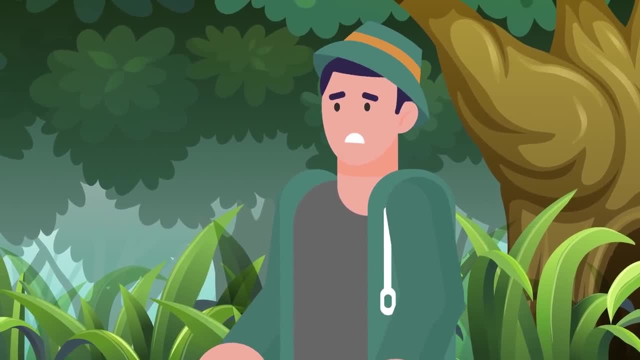 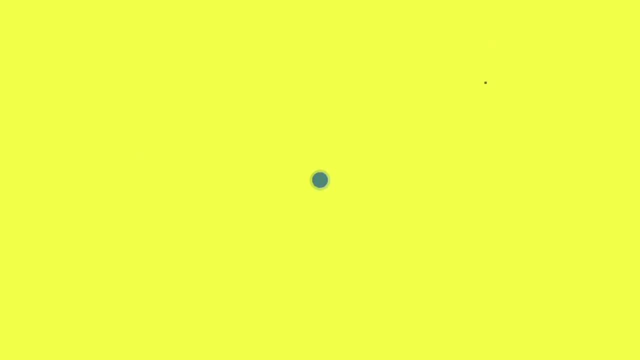 Brazilian Wandering Spiders stand on their hind legs and swing side to side in warning before attacking A bite from this spider causes severe pain at the site of the wound, often with inflammation. Within about 30 minutes, systemic envenomation occurs. characterized by symptoms such as hypertension or hypotension, arrhythmia, nausea, cramping, hypothermia, vertigo, blurred vision, convulsions and paralyzation. If the spider injects enough venom when it bites you, you can die within an hour from. respiratory complications. However, in most cases, bites from Brazilian Wandering Spiders don't contain enough venom to require antivenom. However, victims should immediately seek medical treatment. Even if the spider didn't deliver a fatal dose of venom, it can cause tissue necrosis: 0.006 mg of its venom is enough to kill. 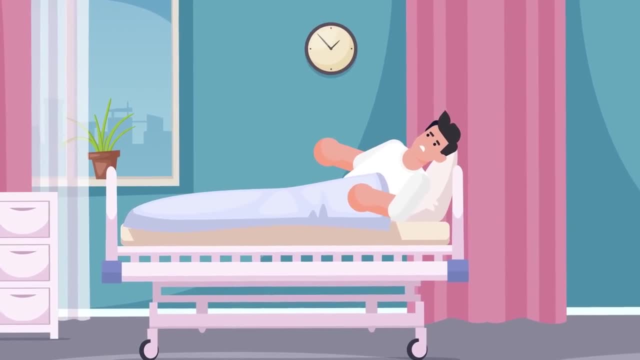 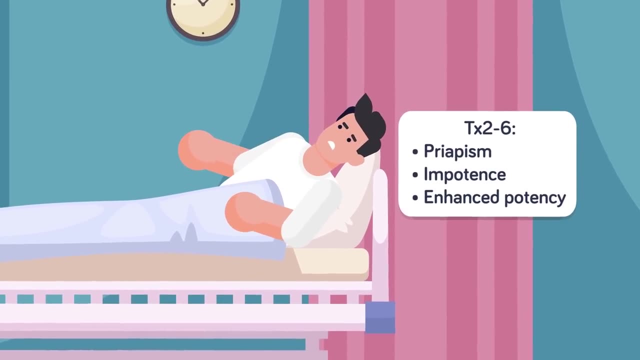 a mouse. Interestingly, the venom of the Brazilian Wandering Spider contains a toxin called TX26 that causes priapism, or long painful erections in males lasting several hours, which can lead to impotence or enhanced potency, depending on the victim. 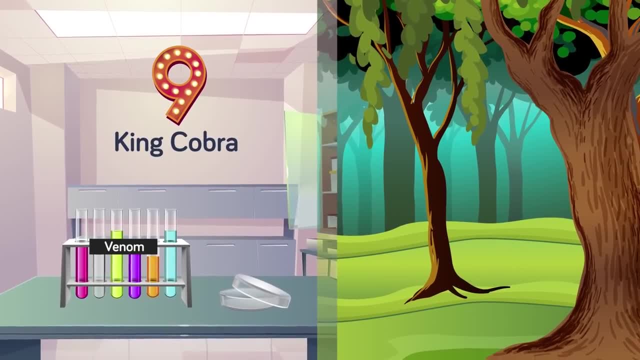 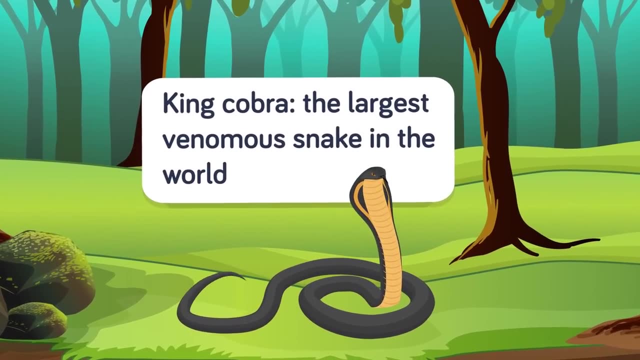 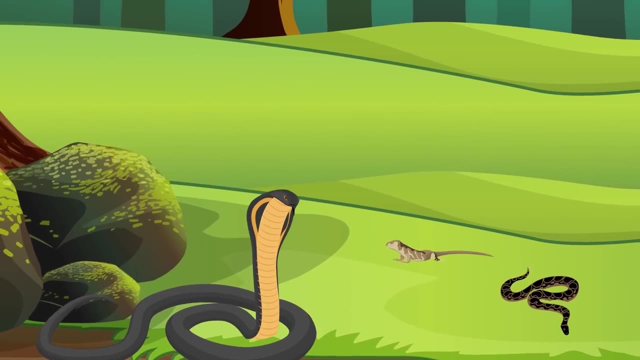 9. King Cobra, Native to South and Southeast Asia, these typically ten to fifteen foot king cobras are the largest venomous snakes in the world. The largest king cobra ever found was just over 19 feet. Generally, their prey is other smaller snakes and lizards which they 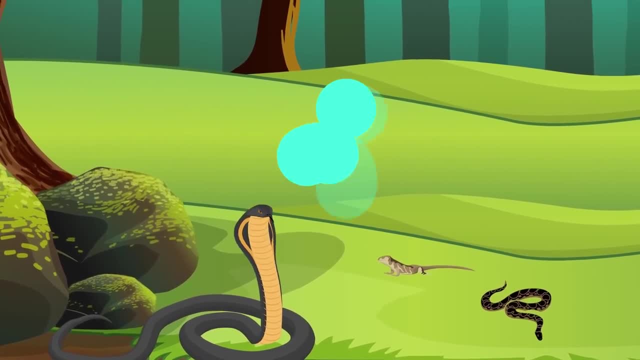 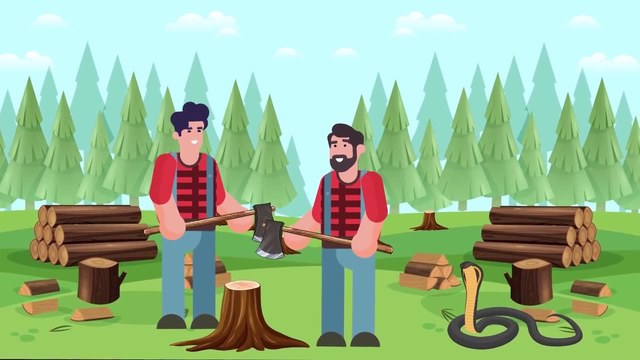 envenomate and then use their flexible jaws to swallow their paralyzed prey whole. Typically, king cobras are non-aggressive and shy, but as their Highland Forests home was encroached on, they are coming into contact with humans more and more. In humans, the risk of death. The king cobra bite is somewhere around 75%. The painful bite can cause the death of a healthy adult human within 15 minutes, although it generally takes 30 to 45 minutes. The king cobra is even capable of killing a full-grown Asian elephant within three hours. 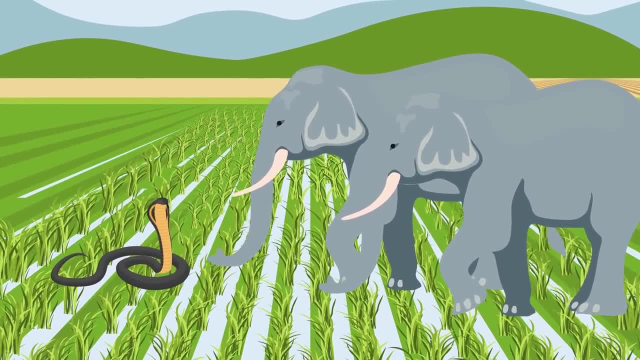 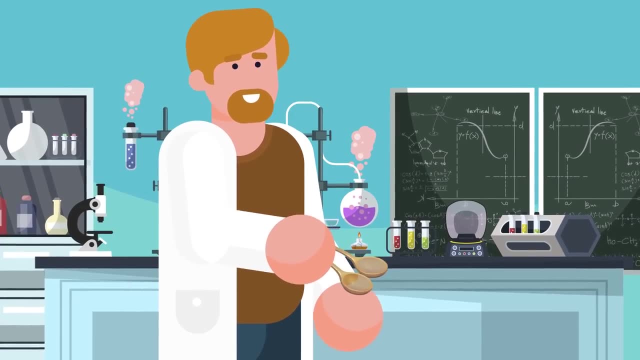 if the pachyderm is bitten in a vulnerable area such as the trunk. Seven milliliters or slightly less than one and one-half teaspoons of a king cobra's venom can kill 20 adult humans or one elephant. 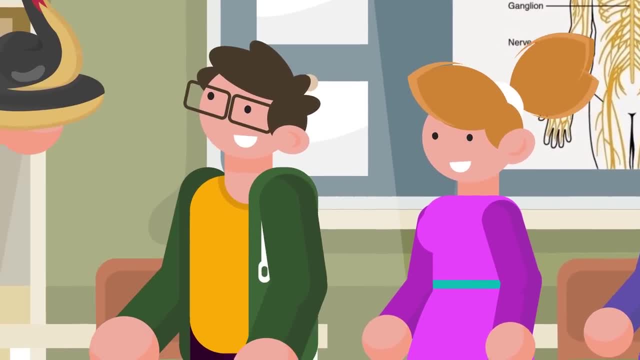 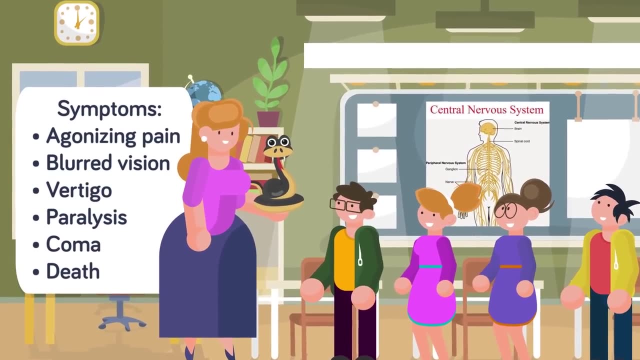 The king cobra's venom attacks the victim's central nervous system, resulting in agonizing, pain, blurred vision, vertigo and eventually paralysis. If the envenomation is serious, it progresses to failure of the circulatory system and the victim falls into a coma, then dies. 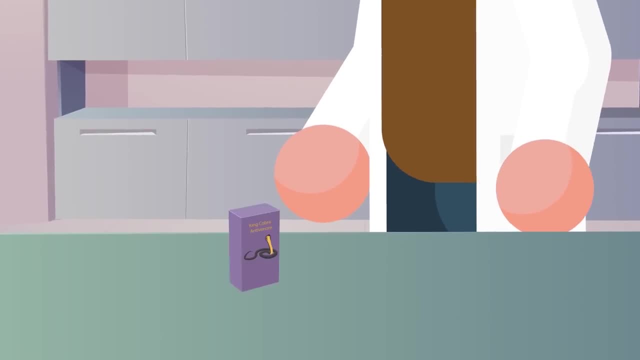 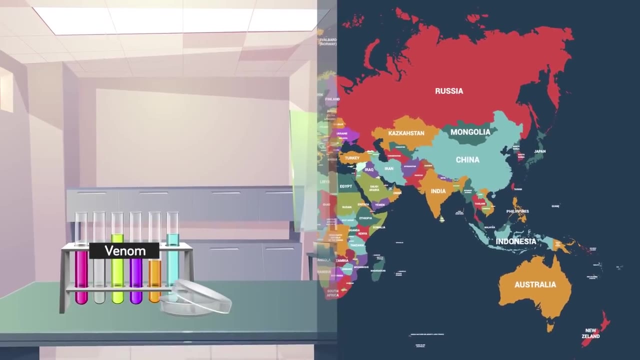 Anti-venom is available in small doses. A traditional Ayurvedic concoction of turmeric and alcohol has also had some success in treating king cobra bite sufferers. Number 8. Sydney Funnel Web Spider. The Sydney Funnel Web Spider is number eight on our list of the most dangerous venomous. 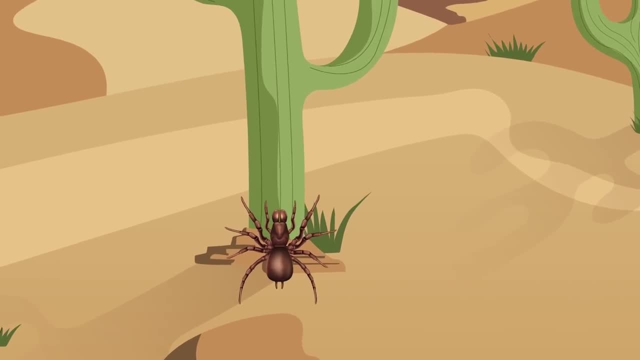 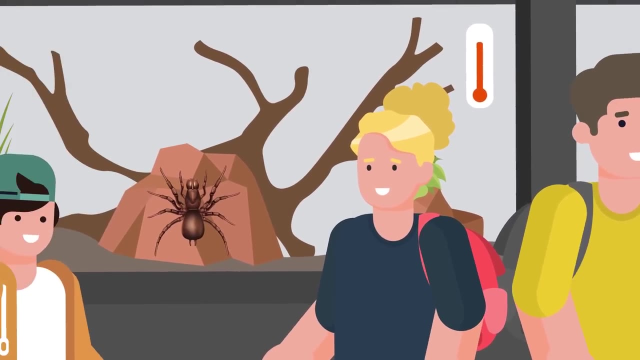 animals in the world. It belongs to a family of approximately 35 spiders native to Australia. Six spiders of the species are venomous, considered dangerous and are known to cause grave injuries to humans. The male Sydney Funnel Web Spider is most likely to come in contact with humans as it 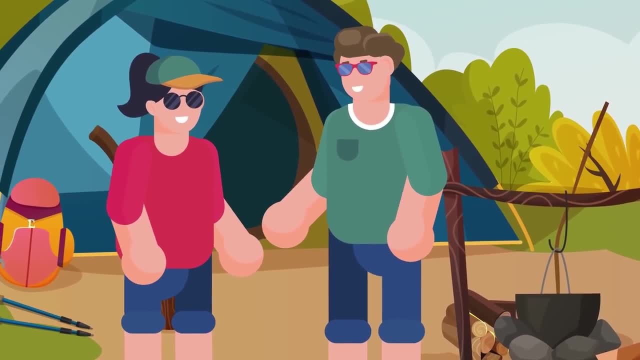 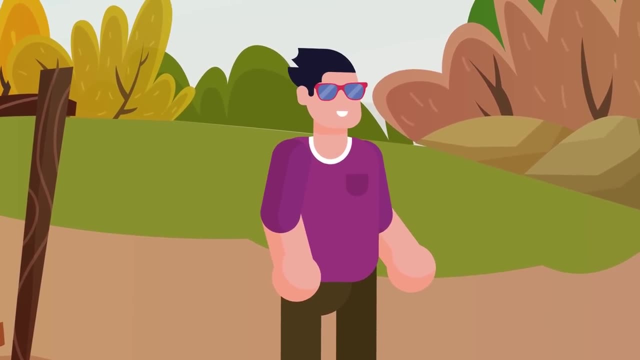 travels to search for a mate. The spider delivers a painful bite with its large fangs and the wound often bleeds. The spider doesn't always inject its victims with venom, but when it does watch out. The venom contains a neurotoxin which it uses to kill. 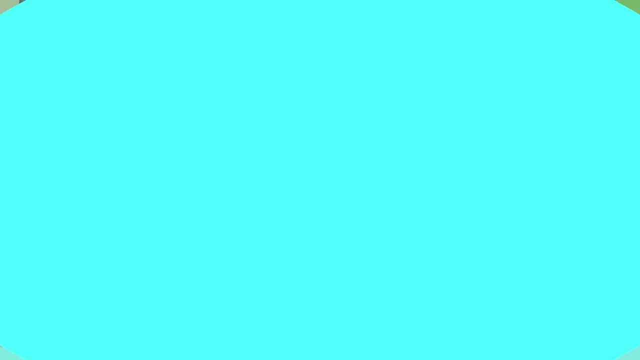 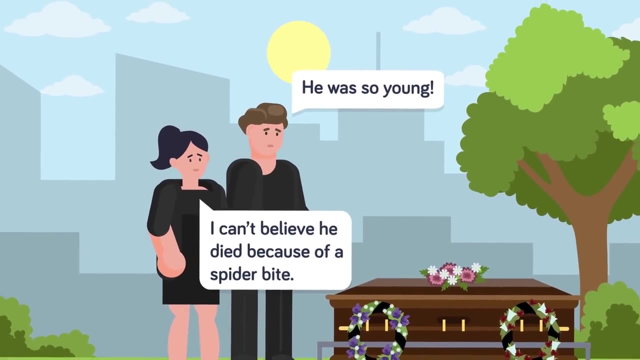 This neurotoxin attacks the nervous system and organs in a human. Fatalities can occur anywhere from 15 minutes in small children to three days for a healthy adult. The venom of this spider is reputedly 60 times as potent as cyanide. Symptoms of envenomation present almost immediately. Early symptoms include sweating, twitching, elevated heart rate and elevated blood pressure As the venom spreads throughout the body. symptoms include nausea, vomiting, muscle spasms, pulmonary edema, metabolic acidosis and extreme hypertension. 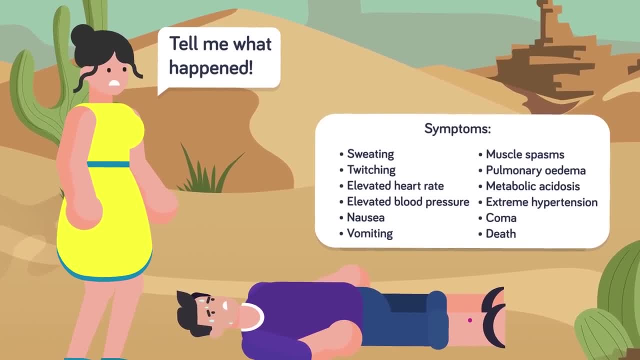 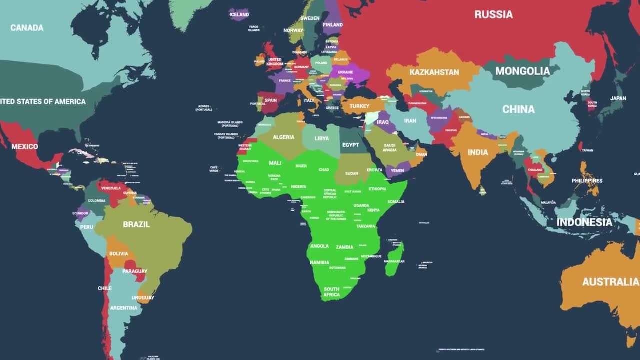 The venom is also known as the sputum. It is a venom that is often used to treat cancer. Often, victims fall into a coma before death. 7. Boomslang: The boomslang is a tree snake native to sub-Saharan Africa. 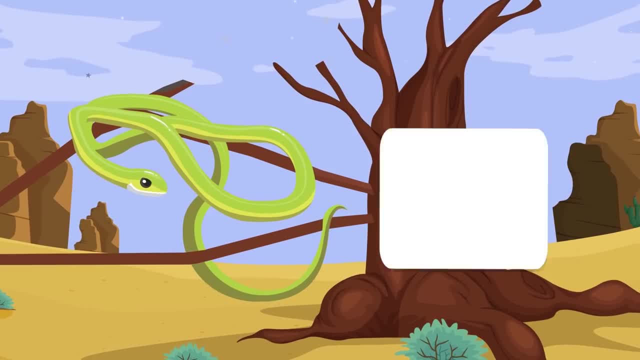 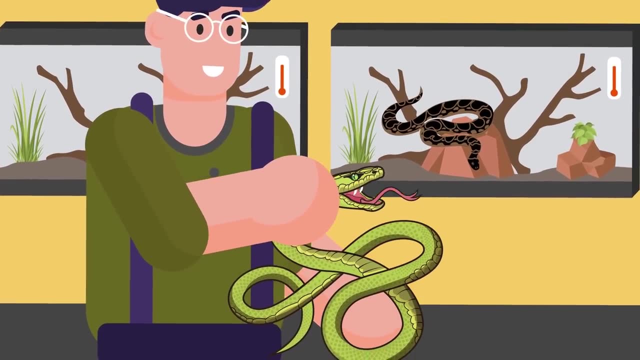 Described as shy and pretty, with large eyes and with a bright light green color in males and brown in females. boomslangs are rear-fanged snakes. Their fangs are far back in their mouths, behind their other teeth, which means to envenomate. 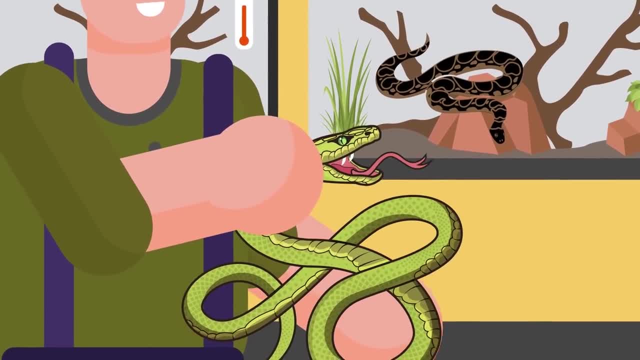 they have to open their mouths really wide, up to 170 degrees, to grab a chunk of flesh and stab When venomously bitten by a boomslang. the snake's mouth will be opened wide and the mouth will be opened wide. 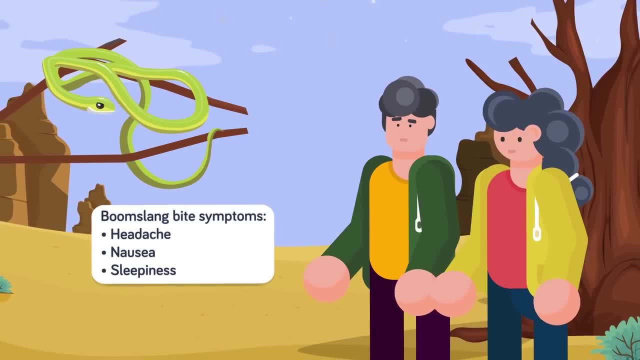 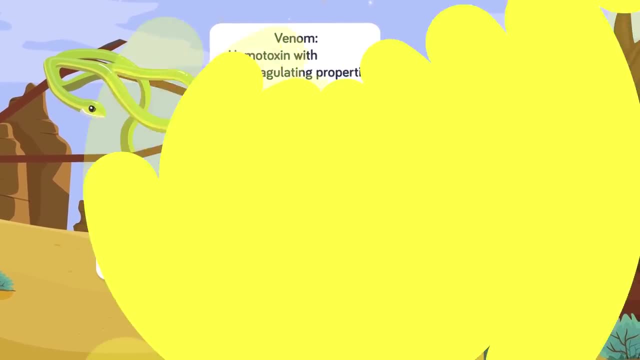 When bitten by a boomslang, a victim experiences several symptoms, such as headache, nausea and sleepiness. However, the most dangerous aspect of boomslang venom is that it is a hemotoxin with anticoagulating properties, In addition to destroying red blood cells, loosening blood clotting and tissue degeneration. 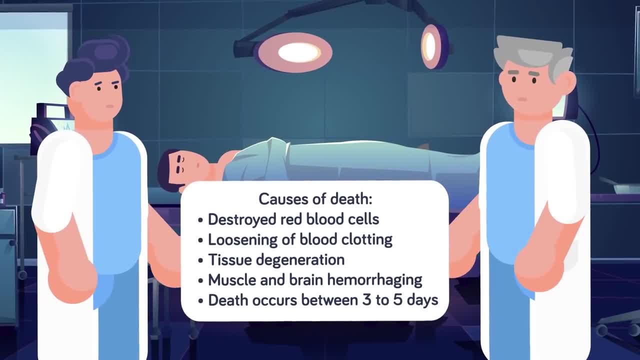 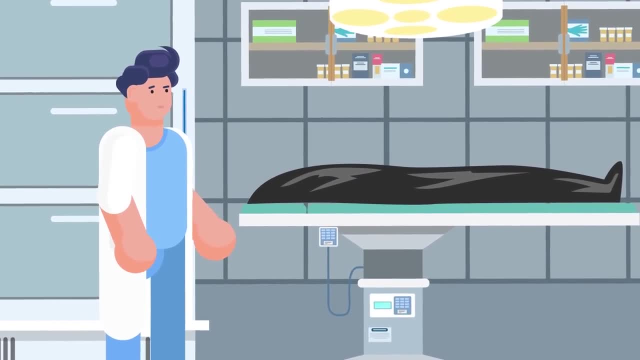 victims suffer extensive muscle and brain hemorrhaging. Death happens via progressive internal bleeding and is a slow, excruciating process taking anywhere from three to five days. It can also be messy and embarrassing. As blood leaks out of a boomslang. the snake's mouth is filled with blood. 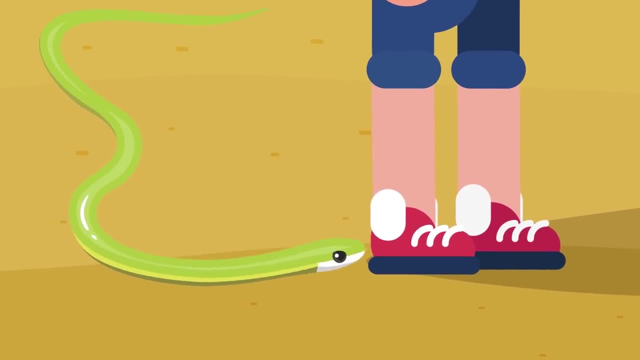 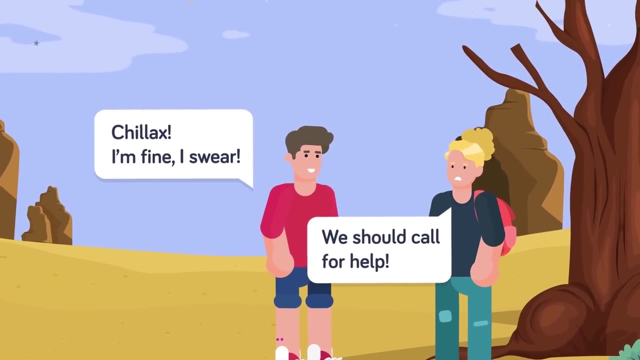 7. Coastal Typhon, Since boomslang venom is slow-acting and symptoms may take several hours to set in. after a venomous bite in the past, victims have been lulled into a false sense of security that the bite was dry or not serious. 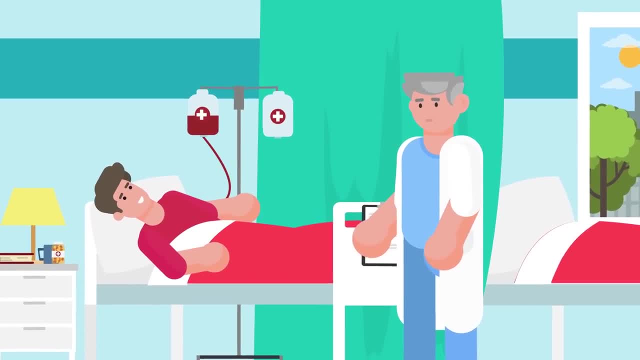 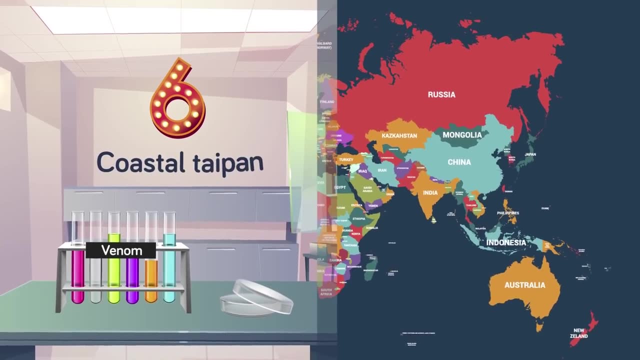 Symptoms may be counteracted with an antivenom and also blood transfusions, depending on the amount of time between the bite and the victim seeking medical attention. 6. Coastal Typhon. The coastal typhon, or common typhon, is native to New Guinea and also the coastal regions. of northern and eastern Australia. Adult coastal typhons typically range in size from 4.9 to 6.6 feet and tend to live in logs, piles of vegetation, and have even been found in trash heaps. Bite victims may experience a wide variety of symptoms, including headache, vomiting. convulsions, paralysis, internal bleeding and kidney failure. In cases of severe envenomation, depending on the health of the victim, death can occur within 30 minutes of being bitten, but on average takes two and a half hours. 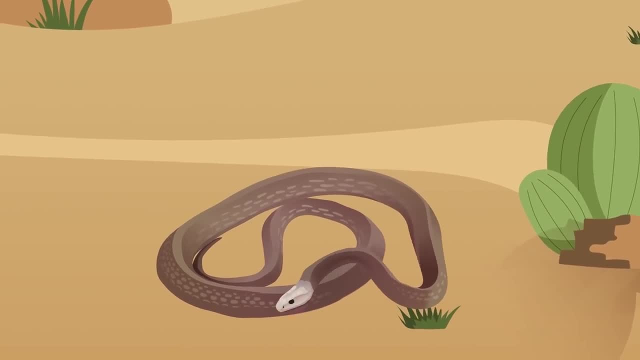 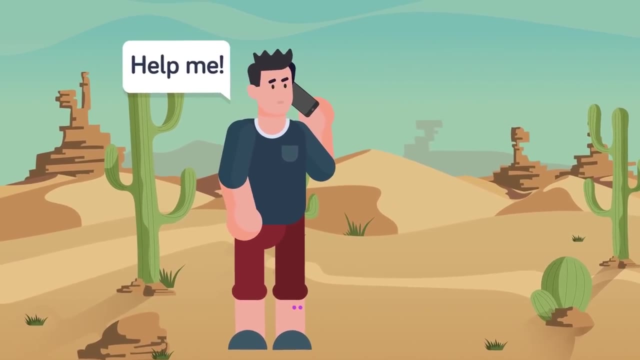 7. Irukandji Jellyfish. The coastal typhon contains a potent neurotoxin which affects the nervous system and the blood's ability to clot. Medical attention must be sought immediately. Untreated bites have a mortality rate of 100%. as the coastal typhon always delivers a fatal 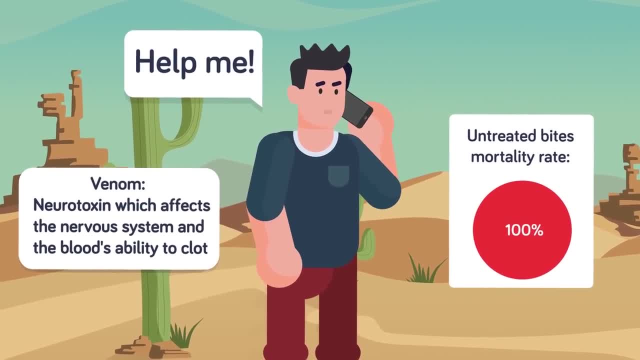 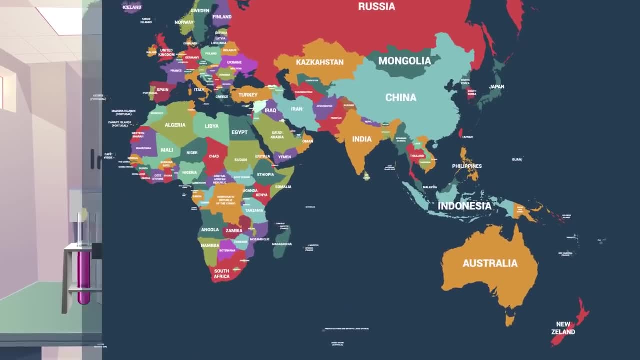 dose of venom. The average bite delivers 10 to 12 times the dose needed to kill a human adult male. 5. Irukandji Jellyfish. Irukandji jellyfish primarily live in the ocean off the coast of northern Australia. 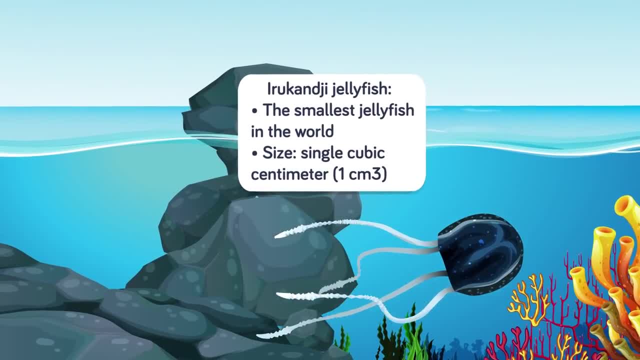 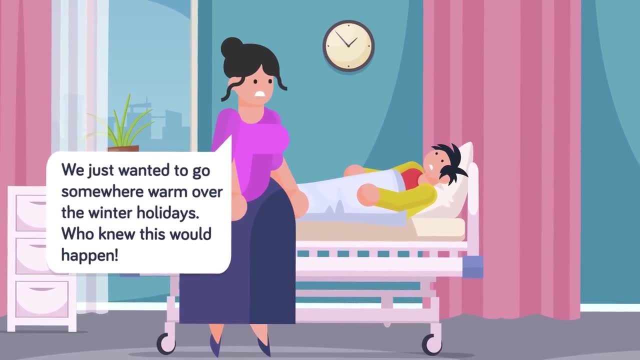 They're the smallest jellyfish in the world. They're the smallest jellyfish in the world. They're about the size of an adult, being a single cubic centimeter. For being so tiny, they are incredibly dangerous. They can shoot stingers into their victim, causing symptoms collectively known as Irukandji. syndrome. While a single sting tends to be only mildly painful, apparently it feels similar to a mosquito bite. The victims are usually struck with multiple barbs and the venom effects aren't immediate. In anywhere from 5 to 120 minutes, with 30 minutes being the average, a victim begins. 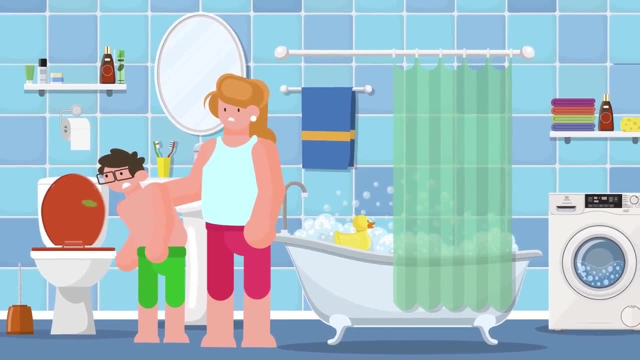 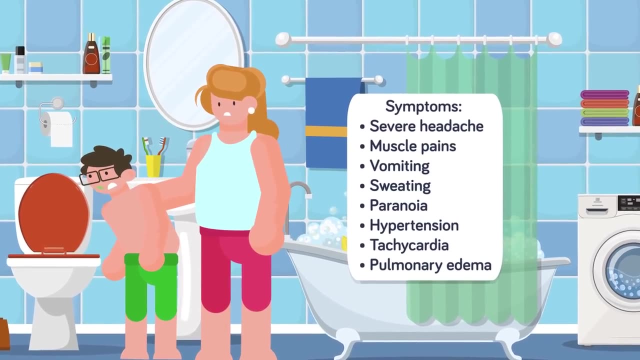 to experience symptoms, including severe headache. 6. Irukandji Jellyfish. Irukandji jellyfish are known to have fatal pains: vomiting, sweating, paranoia, hypertension, tachycardia and pulmonary edema. Thankfully, while often severely painful, Irukandji syndrome is not necessarily fatal. 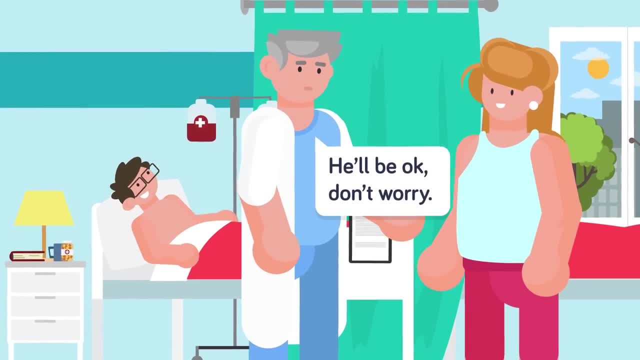 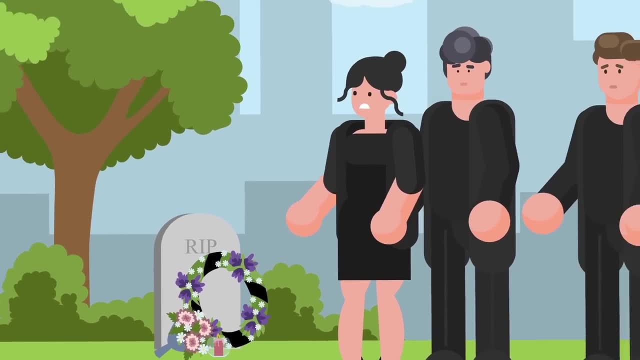 depending on the dose delivered. Symptoms generally improve in 4 to 30 hours, but it may take up to two weeks for a patient to make a full recovery. With a fatal dose, victims often expire within 24 hours of the attack due to brain hemorrhages. 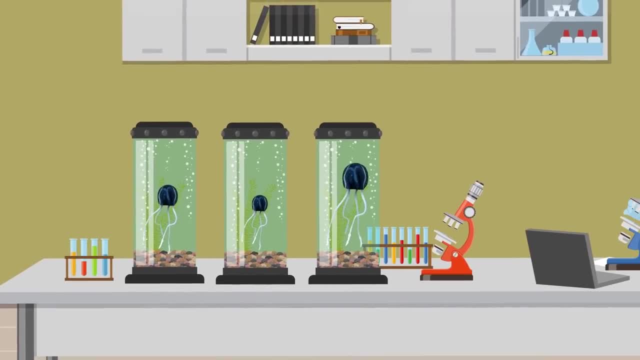 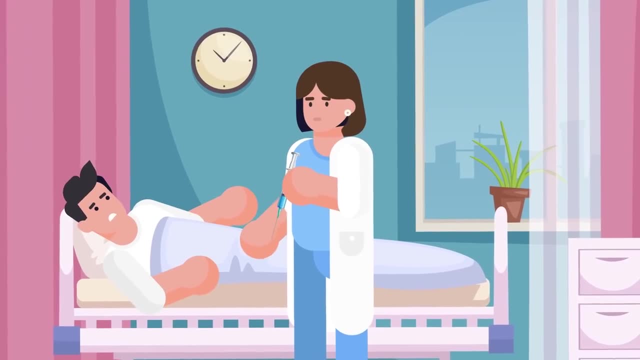 Since Irukandji jellyfish are so tiny and delicate, they've proven hard to study in the hopes of creating a targeted antivenom. Current treatment is symptomatic, such as antihistamines and antihypertensive drugs used to control inflammation and hypertension. 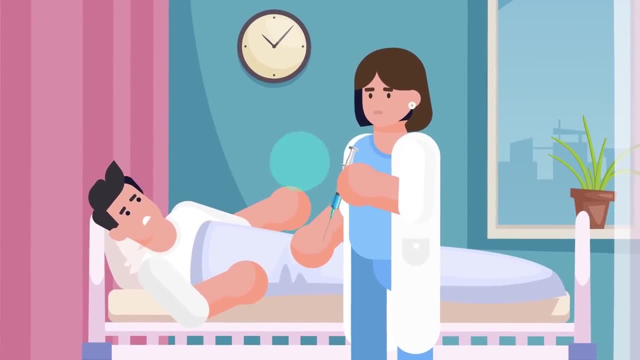 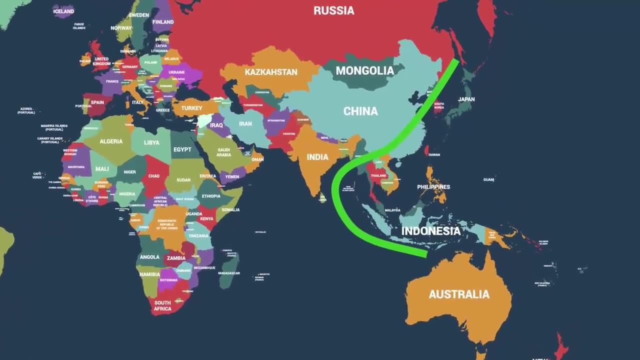 Pain management can be problematic as in some cases morphine has little effect. 4. Blue-Ringed Octopus. The typical adult blue-ringed octopus is about the size of a golf ball and lives off the coasts of Australia and Southeast Asia. 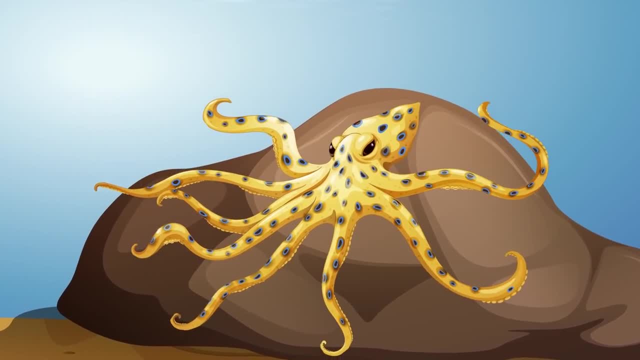 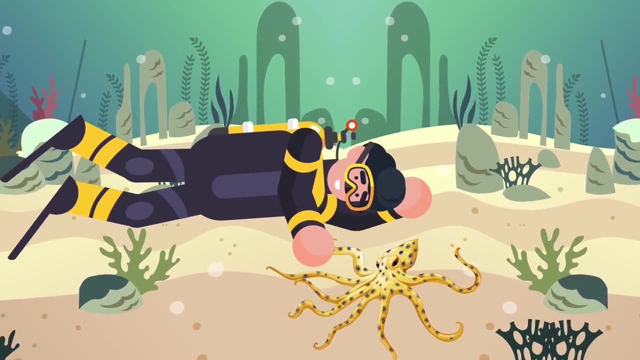 Though usually non-aggressive when provoked, it delivers debilitating and deadly venom for which there is no antidote. The average adult blue-ringed octopus carries enough venom to kill 26 male adults and it's 10,000 times more potent than cyanide. 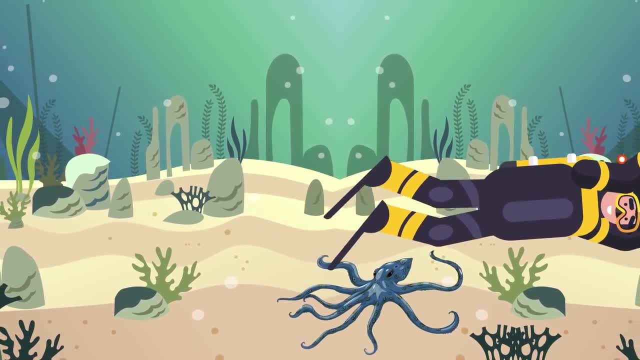 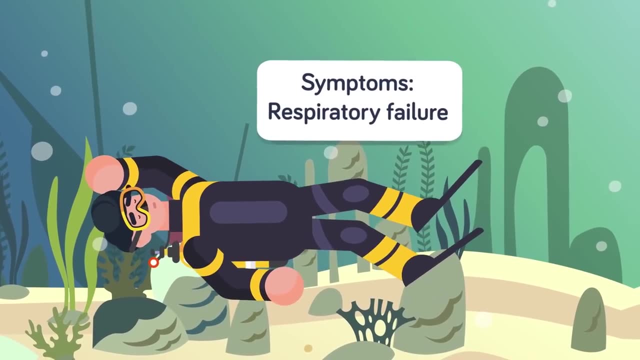 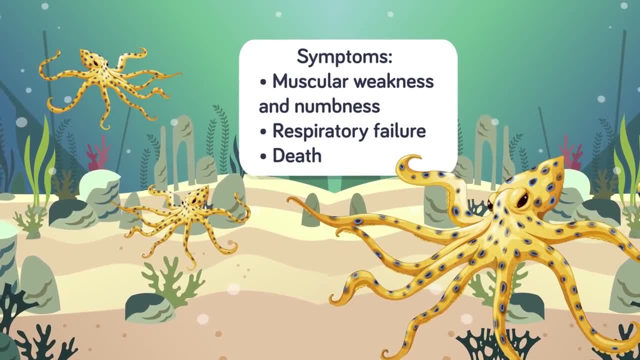 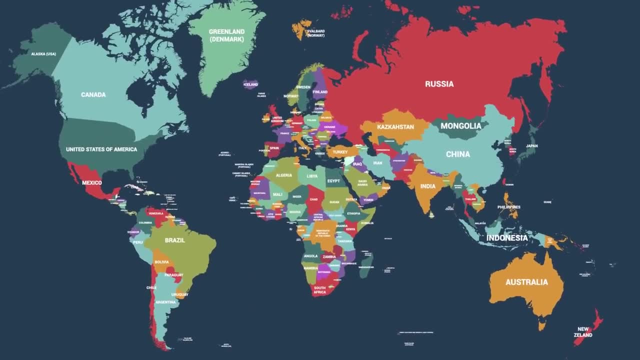 The blue-ringed octopus venom contains neurotoxins which cause the octopus to die. It causes muscular weakness and numbness, followed by respiratory failure and ultimately, death. 3. Inland Taipan. The Inland Taipan, or fierce snake, inhabits semi-arid regions of Central East Australia. 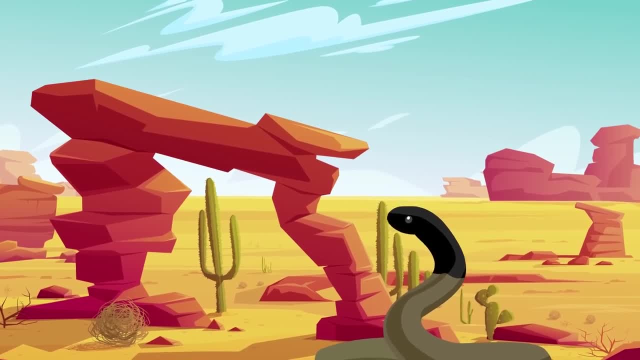 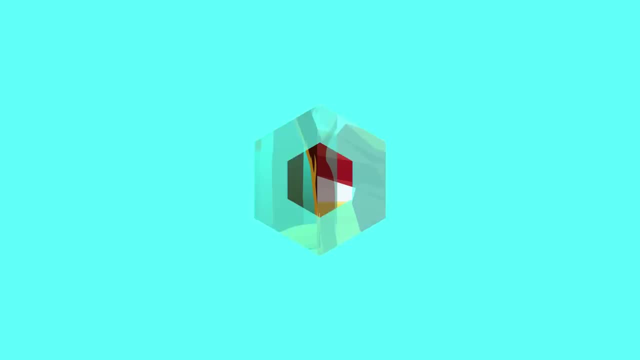 and is considered the world's most venomous snake. It's estimated that one bite is enough of a lethal dose to kill at least 100 male adults or about 250,000 mice. Its venom is considered at least 200 to 400 times more toxic than the common cobra even. 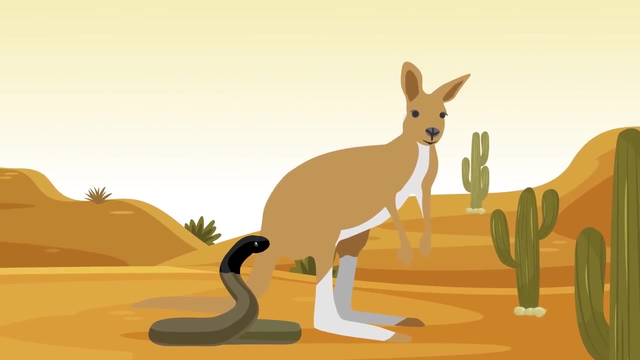 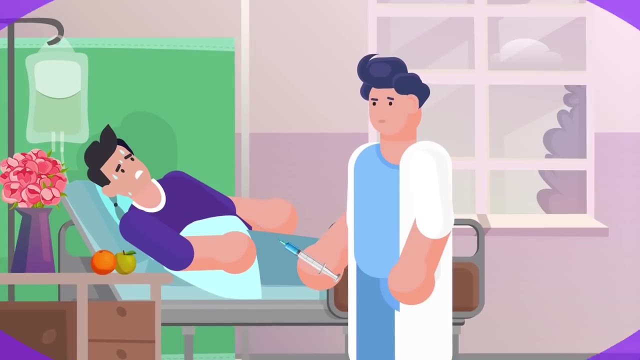 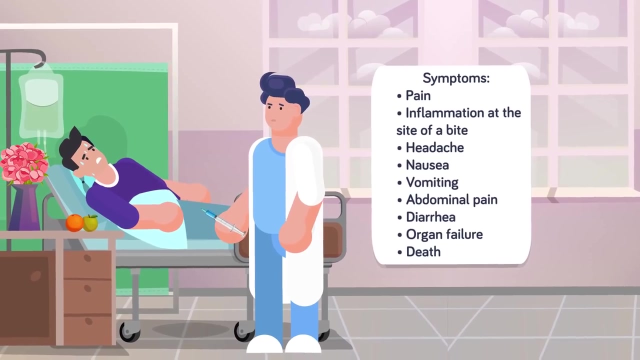 the inland taipan has extreme accuracy when attacking, often striking multiple times in the same attack, and it nearly always injects venom rather than delivering a dry bite. Victims should seek medical attention immediately. If left untreated, an inland taipan bite can kill a human in 30 to 45 minutes, Aside from pain and inflammation at the site of. 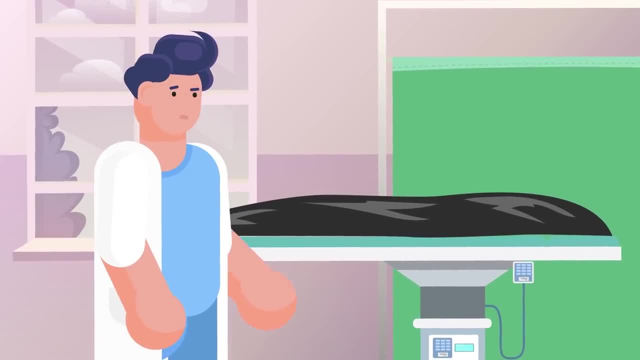 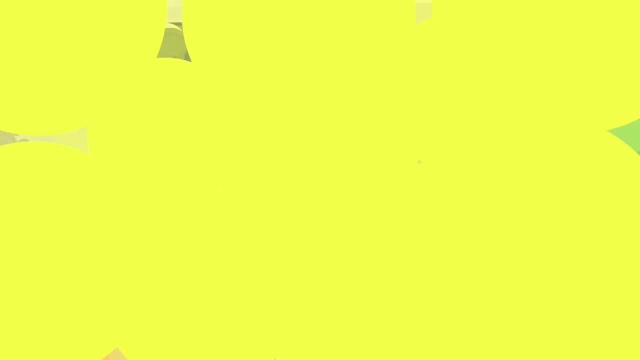 the bite. symptoms include headache, nausea, vomiting, abdominal pain and diarrhea. The victim then collapses or goes into convulsions, leading to major organ failure and finally death. Fortunately, there have been no documented human fatalities from an inland taipan bite. 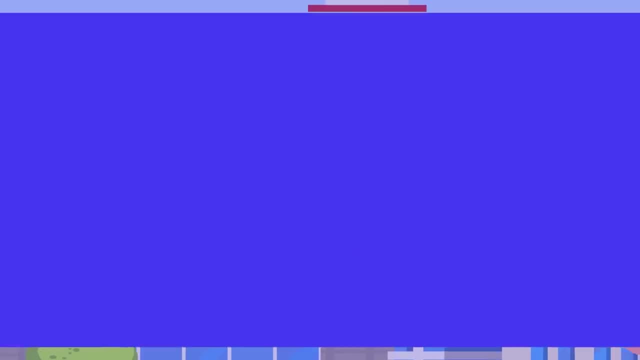 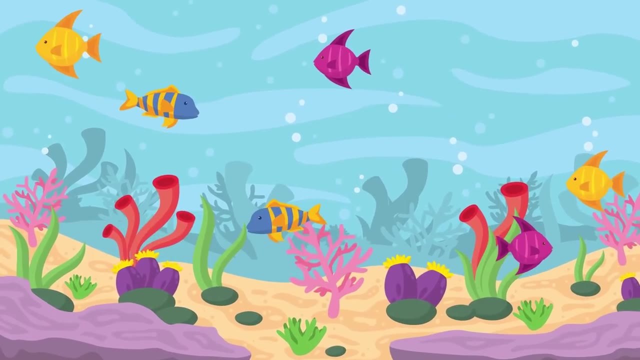 All known bite victims have been successfully treated with antivenom. 2. Cone Snail. The second most venomous animal in the world is the cone snail. The name cone snail encapsulates a family of several hundred species of marine gastropods. All of them are extremely venomous. 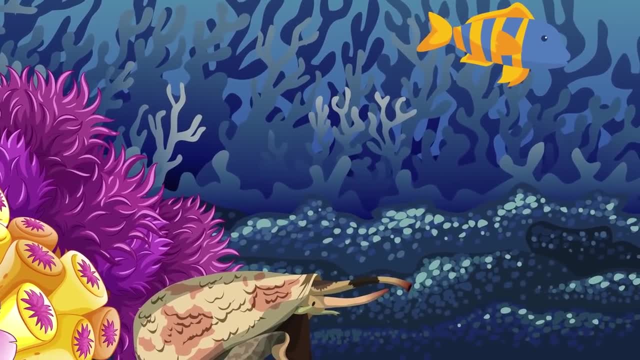 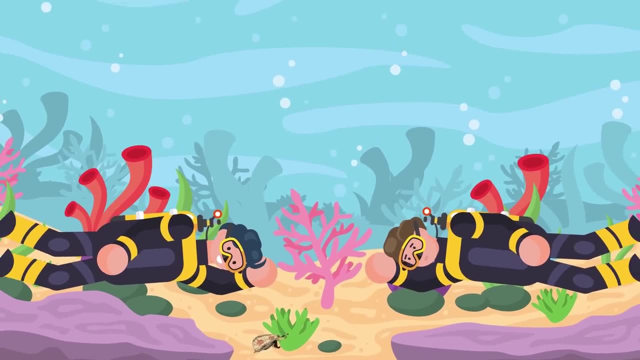 and dangerous to humans. They typically live in tropical cities such as the United States. the United States and the United States. Cone snails live in the middle seas, in the sand or among coral reefs and rocks. They move slowly. Their venom is used to capture prey. Fortunately, they can be easily avoided If 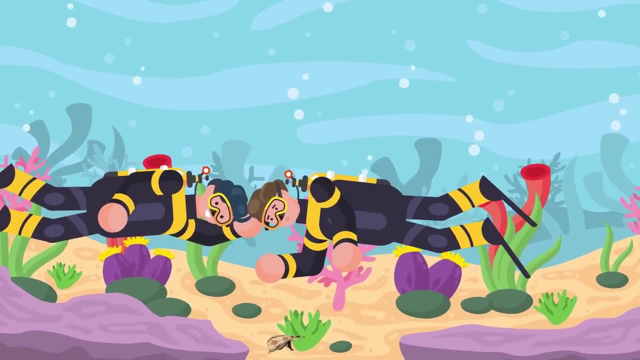 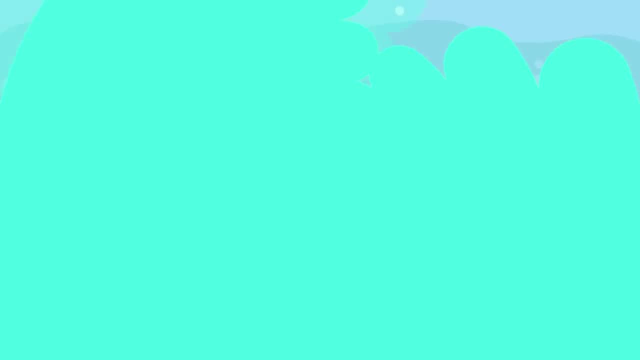 you're foolish enough to pick up a live cone snail, you may be courting death. They shoot harpoon-like sharp teeth from their mouths to sting and then pump venom into their victims via muscular contraction. The harpoon of a large cone snail can even penetrate wetsuits. 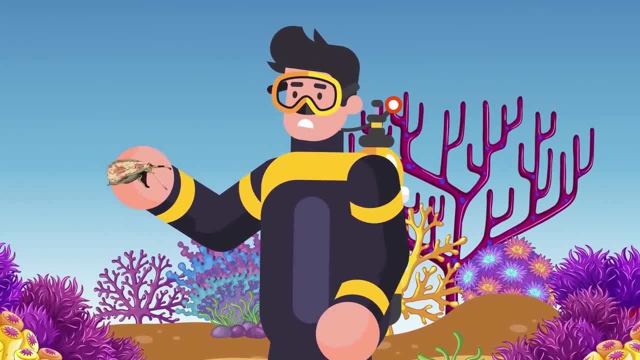 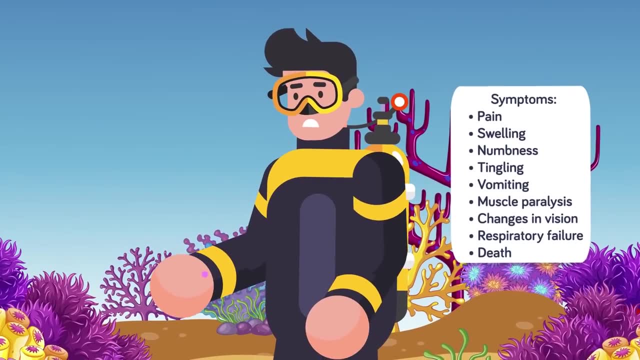 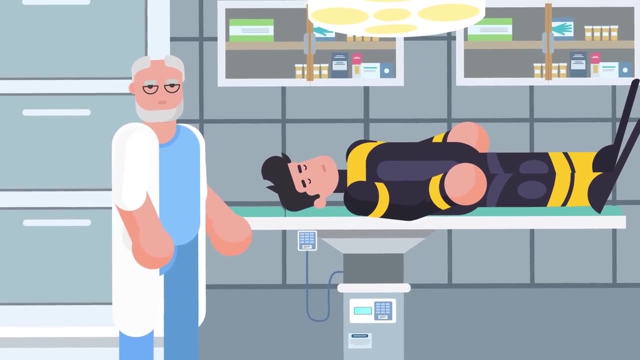 Intense pain at the site of the sting is often immediately felt, followed by swelling, numbness, tingling and vomiting. Severe cases, rapid paralysis, changes in vision and respiratory failure can lead to death. The venom of larger cone snails can potentially kill a human in four minutes. though it generally takes longer, A venom dose fatal to humans is incredibly small. It's thought that the venom in one cone snail is enough to kill twenty adults. Researchers are studying some species of cone snail in order to harness the toxins to create. 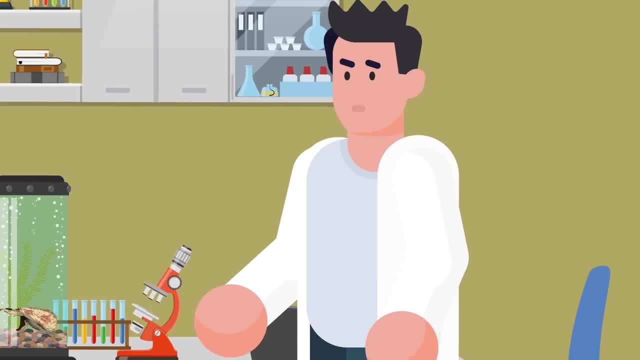 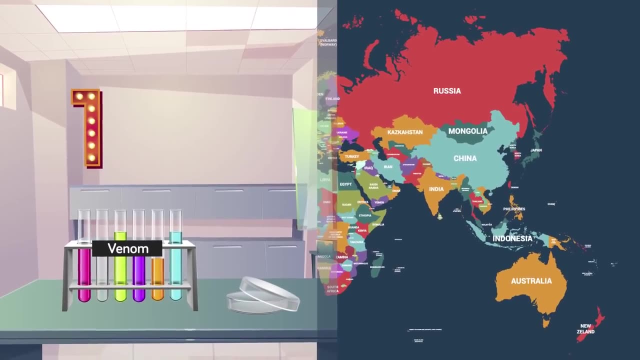 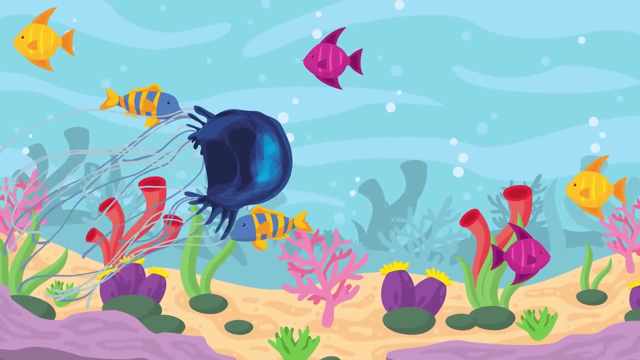 various pharmaceutical drugs. A chemical extracted from the venom of the magical cone snail is a pain killer one thousand times more potent than morphine. 1. Australian Box Jellyfish. The world's most venomous animal title goes to the Australian Box Jelly. It's one of the world's 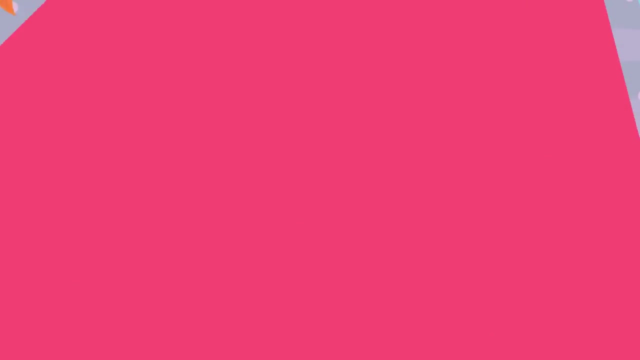 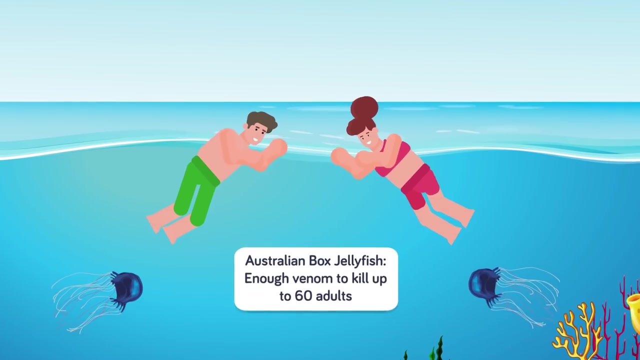 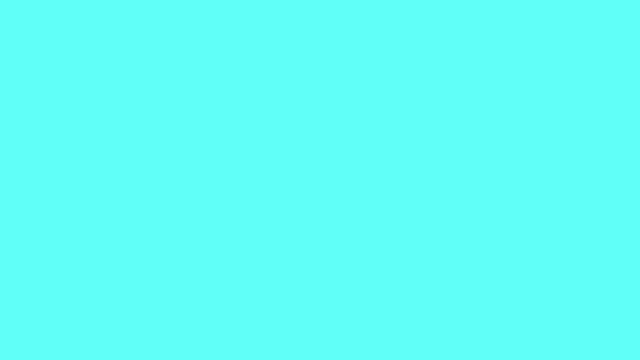 most deadliest animals, as humans fairly frequently come into contact with them. Since jellyfish aren't really fish, biologists have dropped the fish part from its name. No matter what you call it, if an Australian Box Jelly stings you, you're having a really, really bad day. It carries enough venom to kill sixty adults. 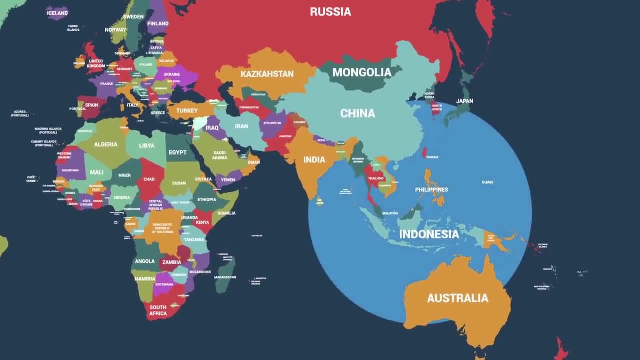 The Australian Box Jelly is the world's most venomous animal. It's the world's most venomous animal. This species of box jelly can primarily be found in the oceans around Asia and Australia. Box jellies are virtually transparent in the water. Adults can measure up to about twelve. 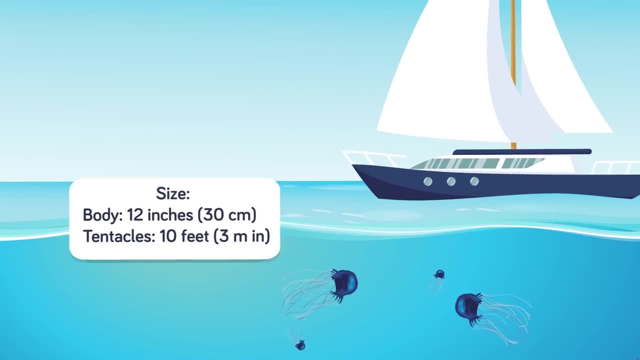 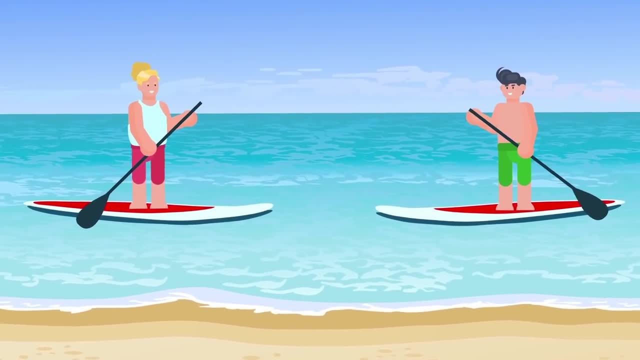 inches in diameter in the box or bell-shaped core body, and the tentacles can grow nearly ten feet in length. Each box jelly has around fifteen tentacles on each corner of its box. Each tentacle has about five thousand nematocysts or microscopic harpoon-shaped barbs.